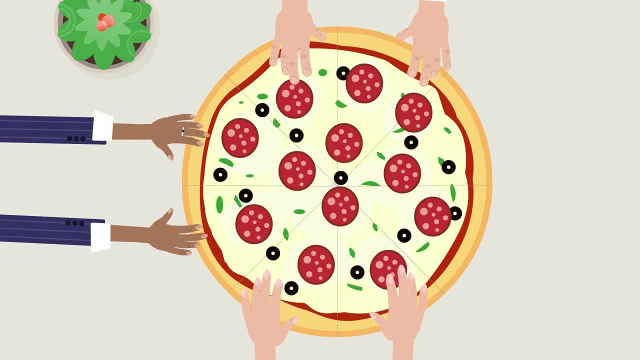 Yay, It's time for pizza. This is awesome. Look, Sarah, you have pizza all over your hands. Now you have to wash it. La-la-la-la-la-la-la-la-la-la-la-la-la-la-la, la-la-la-la-la-la-la-la-la-la-la-la-la. 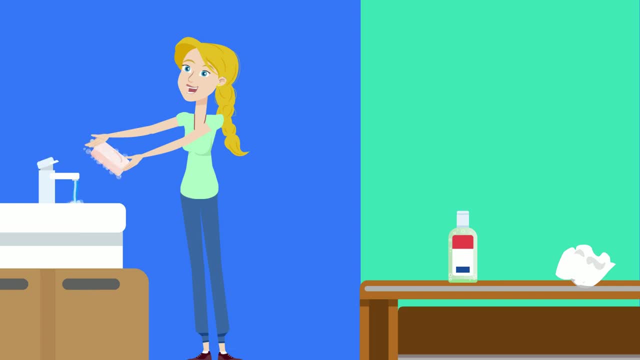 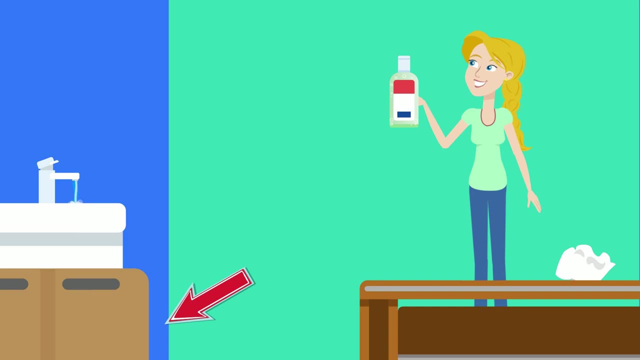 As I wash my hands for twenty seconds and sing the birthday song, Oh look what I found: a chemical from underneath the sink. I know I'm not supposed to go in there and play with things, but this looks so interesting. Yesterday Guys, what should Sarah do? 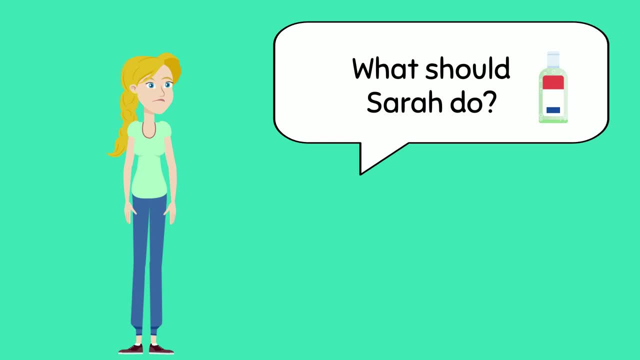 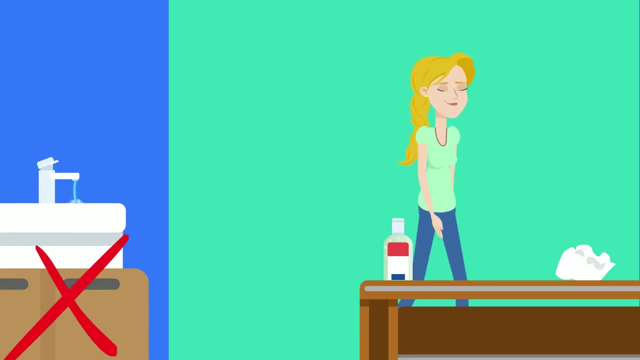 Should she play with the chemical that she found underneath the sink? What is the right thing to do and what is the wrong thing to do? Help her out. You guessed right: Sarah's leaving the chemical alone and walking away so that she doesn't do anything dangerous. 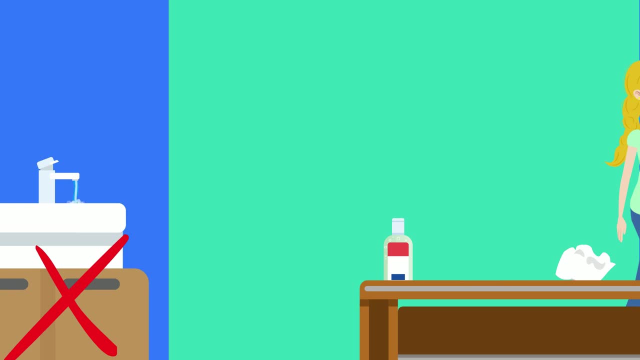 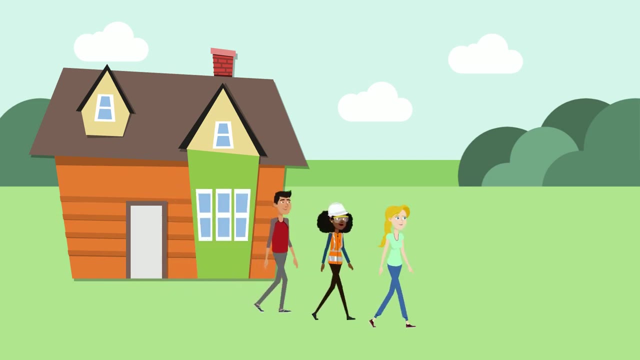 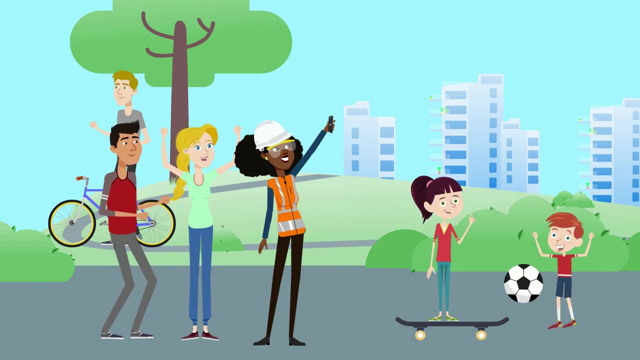 Never play with chemicals underneath the sink. Always ask an adult for permission first Time to go to the park. Let's have some fun. Oh yeah, TikTok time. Come on, let's make a video. This is going on my TikTok today. 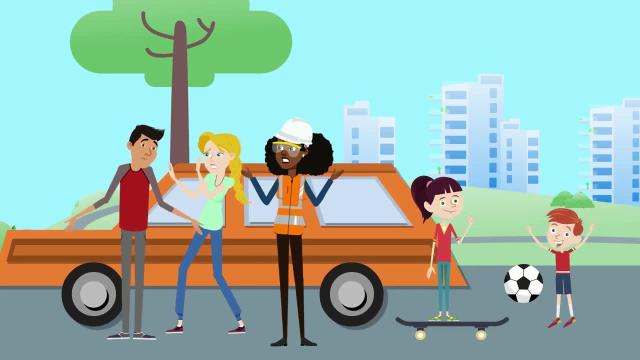 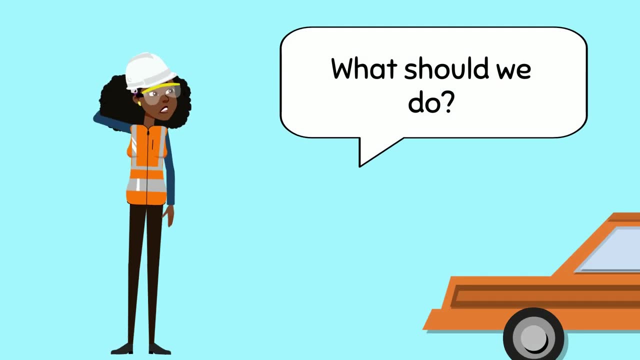 Ryan and Sarah, do you see that weird car slowing down near us? It's a stranger trying to talk to us. What should we do? Should we talk to the stranger or ignore the stranger? What is the right thing to do or the wrong thing to do? 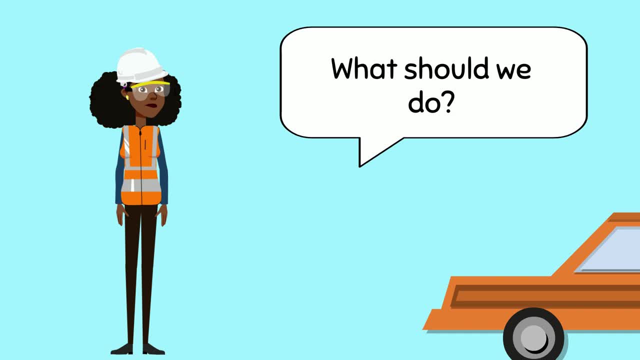 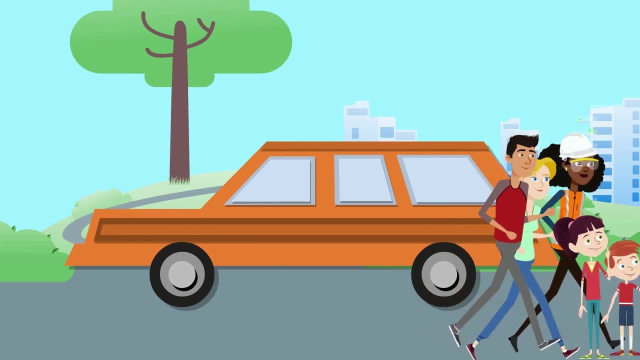 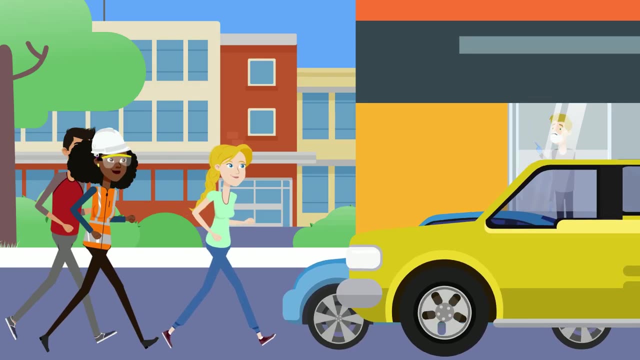 Help us decide. You guessed right: Stranger danger, Stranger danger. The right thing to do is to get out of here and quickly go tell an adult Time to head home. Slow down, Sarah, There are cars ahead. What should we do? 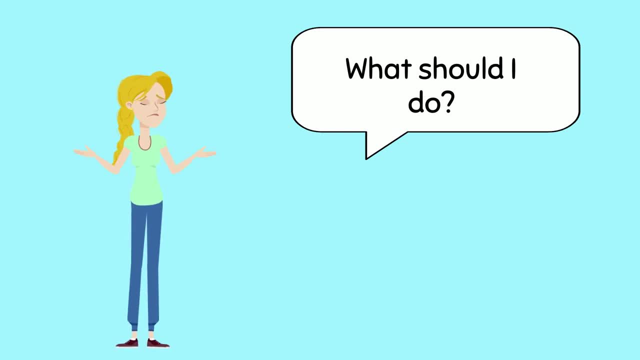 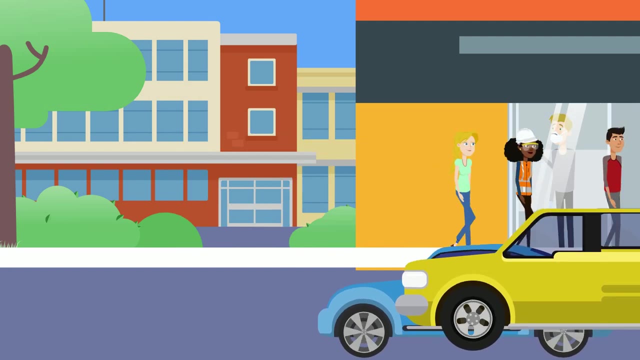 Should I continue to run in the street so I can get home as quickly as possible? What is the right thing to do and the wrong thing to do? Guys, help me out. You guessed right: We will walk on the sidewalk so we do not get hit by a car.